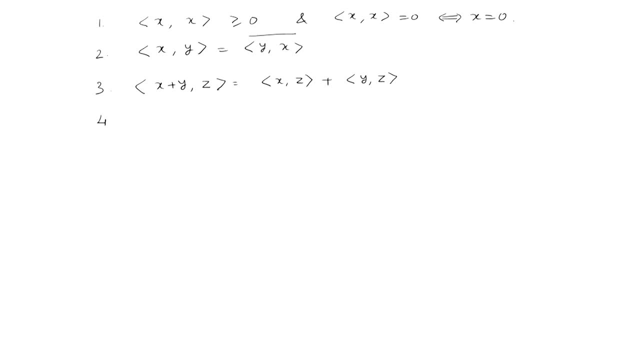 inner product of y, z And the fourth property is: So: the fourth property is Inner product of inner product of alpha. x comma y is same as inner alpha times, inner product of x comma y, where alpha is any scalar in field. So if you have a function in which 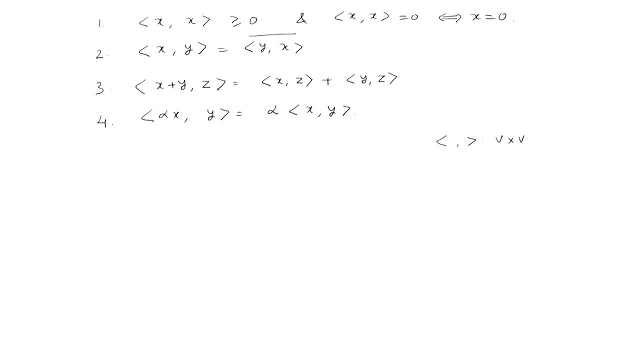 is defined like this: from v, cross v to f, satisfying these 4 properties, then that product is called inner product. ok, And that vector space defined. Now one important property which can be seen from the 4th property. you see, if you take inner product of x, comma, alpha y, So that will. 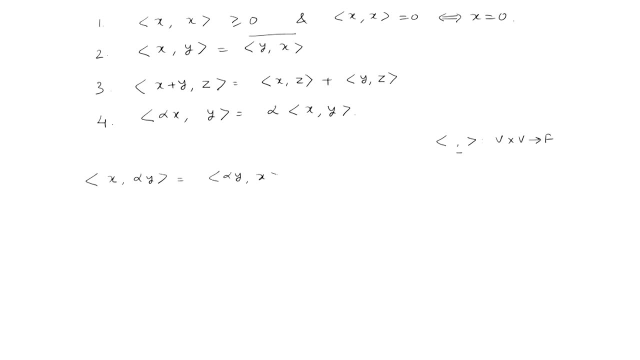 be equal to inner product of alpha y comma x whole bar by a second property, So this can be written as using this property. this can be written as alpha times: inner product of y x whole bar which is equals to alpha bar, and the inner part of y comma x whole. 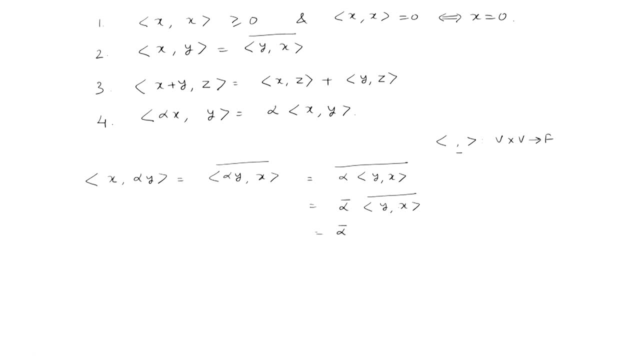 bar and this alpha bar and the inner part. the complex conjugate of this from the second property is equals to inner part of x comma y. So if this scalar is in the second with the second component, then it is alpha bar, and if it is a first component, then it is. 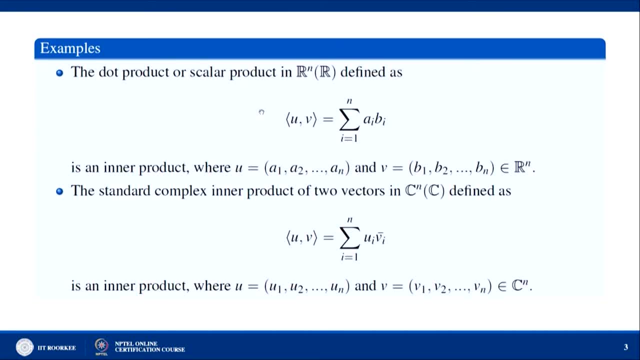 alpha. Now let us discuss first few examples based on this. the first is: example is the dot product in R n. If you define a dot part in R n which is defined as this, then this is the inner product. space defines the inner product. Let 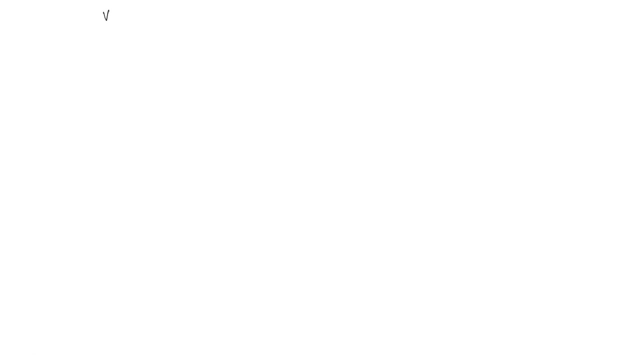 us see how You see you are taking v as R n and field as R. and if you take u as A 1, A, 2 up to A n and v as R n and v as b 1, b, 2 up to b n, then the inner port of u and v is simply summation of a, i. 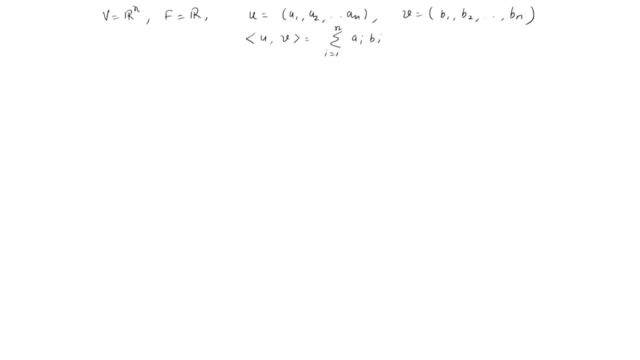 b i i from 1 to n. Now this can easily be shown. you see, the first property is inner port of u comma u. what the inner port of u comma u? it is summation i from 1 to n a i into a i, which is simply summation i from 1 to n, a i squares, or a 1. 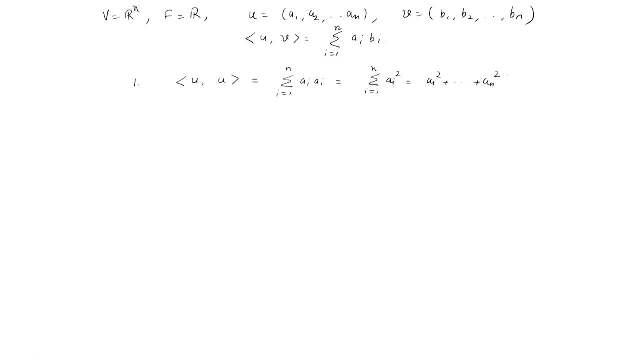 square plus a 2 square, up to a n square, and that is always greater than equal to 0. And this inner product is equal to 0 if, and only if. you see, if it is equal to 0, this implies sum of a i is equal to 0.. 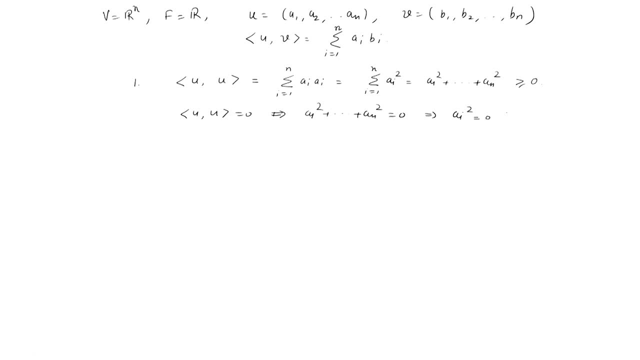 So a i equal to 0 for all i, a i equal to 0 for all i, and this means u equal to 0, and of course, if u equal to 0, then this implies inner port of 0. comma 0 is of course 0 by. 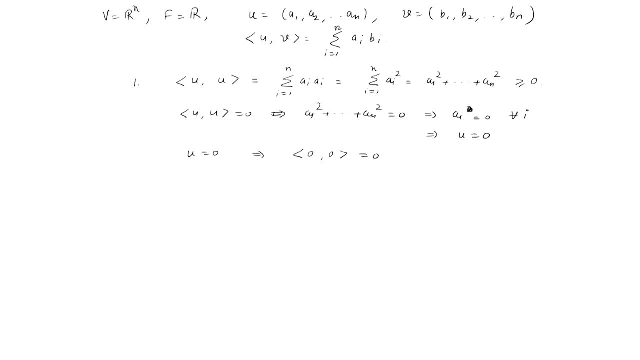 this definition. So the first property holds. Now for second property. you can see inner product of u comma v. if you write it is a 1, b 1 plus a 2.. So this can be written as b 1, a 1 plus b, 2, a 2, and so on up to a, n, b n. this can be written: 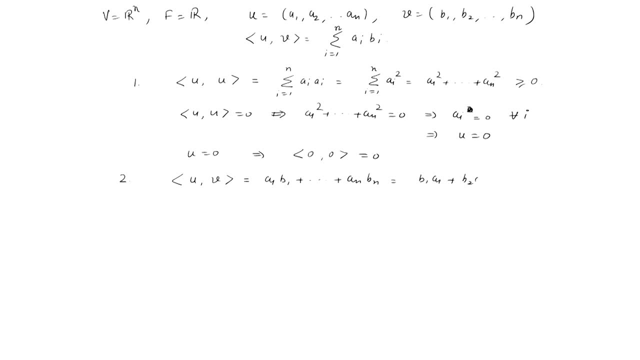 as b 1, a 1 plus b 2, a 2 and so on up to b and a n. So this is same as inner port of v comma u, because we are talking in real space. I mean real field, it is a real vector space. So 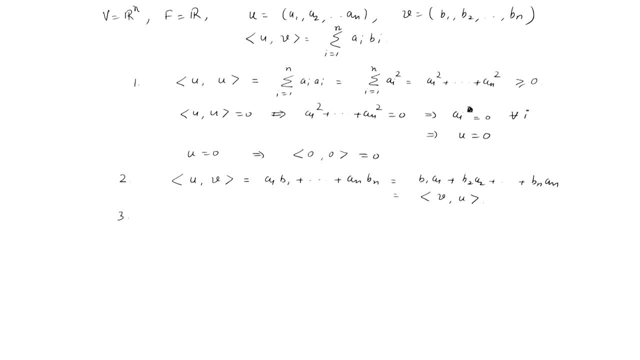 bar. it is itself. Now the third property is. third property is inner port of u comma, of v comma u plus v comma w is equals to. you can see: if you take w as c, 1, c, 2 up to c n, then this will be equals to summation i from 1 to n. it is a i plus b i times c i by this. 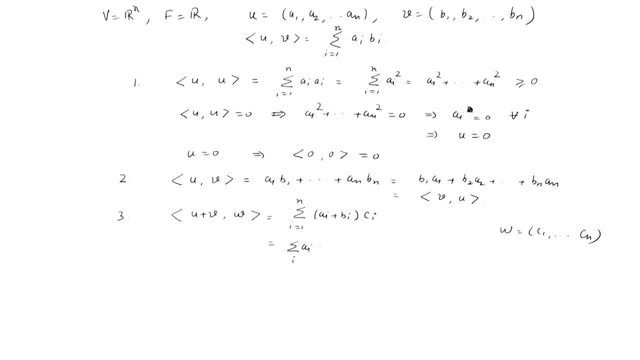 definition, which is summation over i, a, i, c, i, plus summation over i, b, i, c, i, and this is equal to inner product of u and w plus inner product of v and w. So third property also holds. Now the fourth property is inner product of alpha times u. 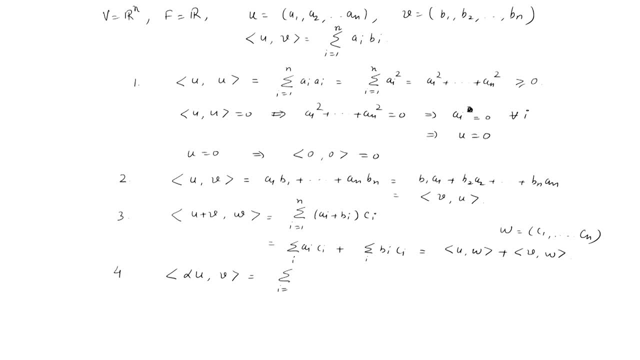 comma v is equals to. this is summation i from 1 to n. So it is alpha times a, i, b, i and, as you can already see, and this is equals to alpha times, summation i from 1 to n, a, i, b, i, which is equal to alpha times inner product of u comma v. So hence we have seen that. 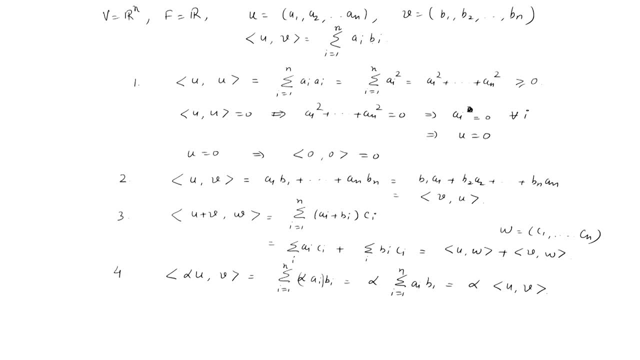 all the 4 properties hold over this definition. when we define the inner product by this, all the 4 properties hold. So this defines inner product and the vector space over which this inner product is defined. we are calling that vector space as inner product. 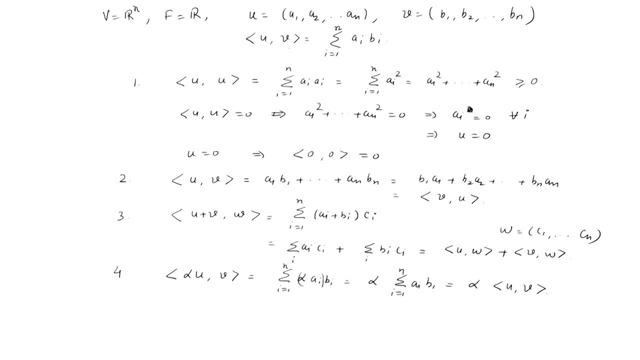 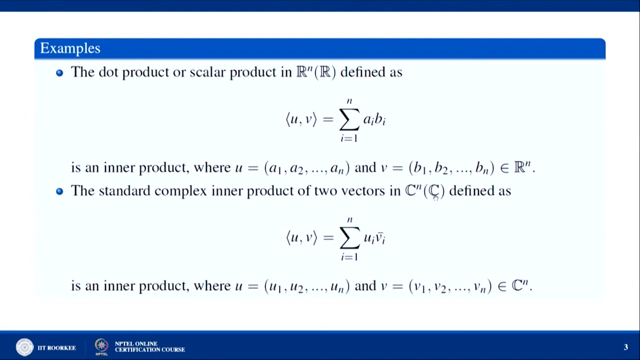 So there may be some other ways also to define the inner product over R n. this is, this is one of the way we are defining the inner product between u and v. Now, if you take c n- I mean vector space- as c n over the complex field, then the inner product may be defined like: 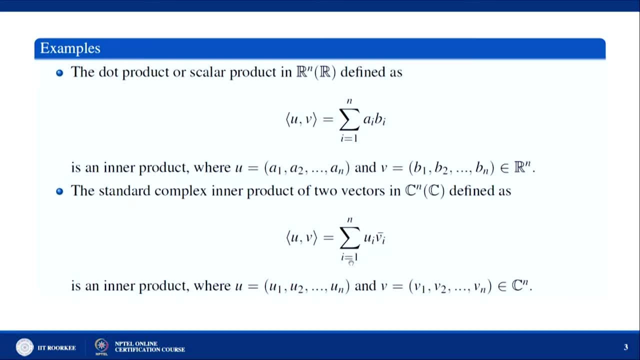 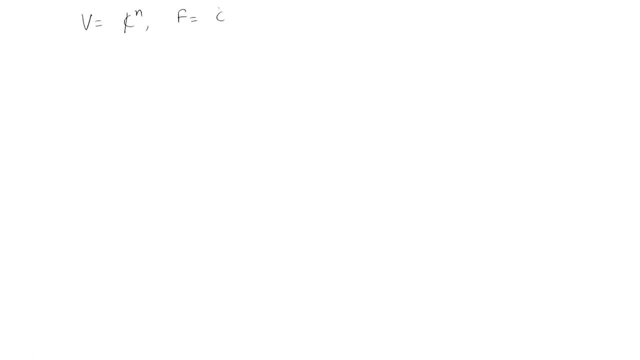 this. ok, This is again formed the inner product. this can easily be verified. you see, if we are taking v as c, n And field as c, ok, now inner product of u and v for any u v in c, n is defined like this: i from 1 to n, it is u, i is v, i is bar conjugate of this. ah, we are. we are taking u as u, 1, u. 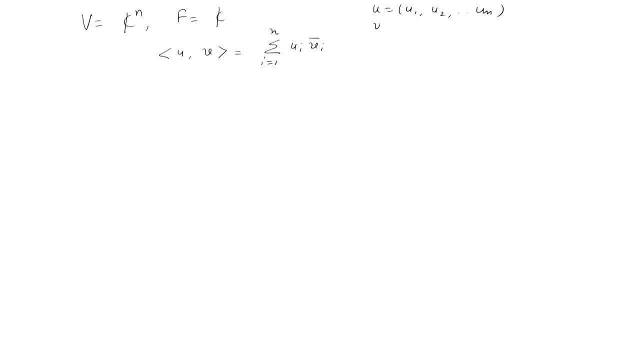 2 up to u n and v as v 1, v 2 up to v n. ok, So the first property is that t is equal to that inner product of u comma u. it is equals to summation over i, u, i into u i bar which. 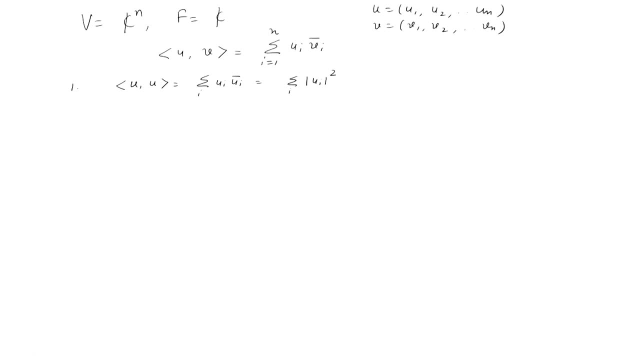 is summation over i mod of u i squares. This means mod of u 1 square plus mod of u 2 square and so on up to mod of u n square. So this is always greater, equal to 0 for all u Now. 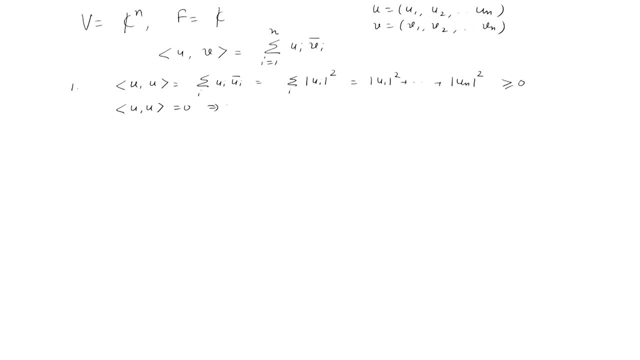 if this is equal to 0, this implies mod of u 1 square plus, and so on. mod of u n- equal is equal to 0, and this implies mod of u n is equal to 0 for all i, and this implies u i equal to 0 for all i, and that means u equal to 0.. 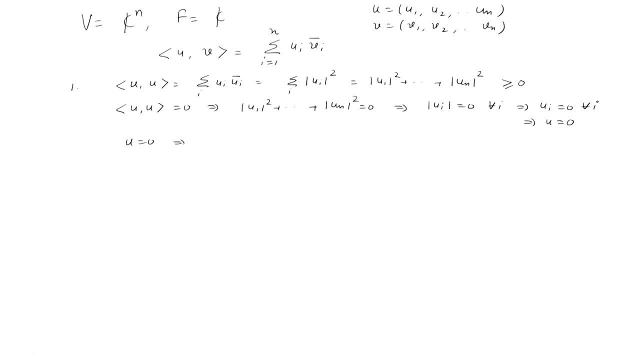 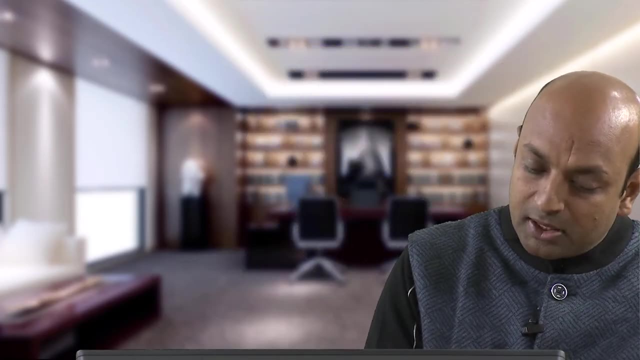 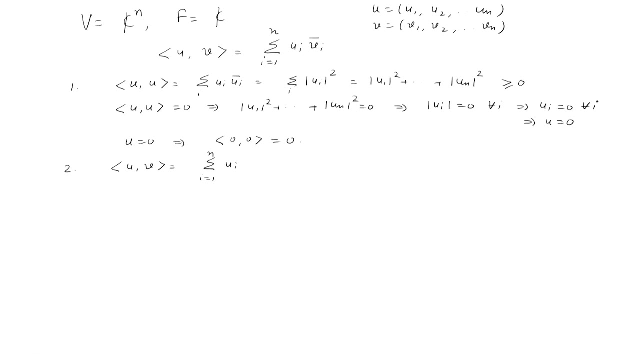 Now, if u equal to 0, of course inner product of 0 comma 0 is 0. So the first property holds. Now for second property. inner product of u comma v, if you take, is summation i from 1 to n? u i v i bar, which can be written as summation i from 1 to n v i u i bar whole. 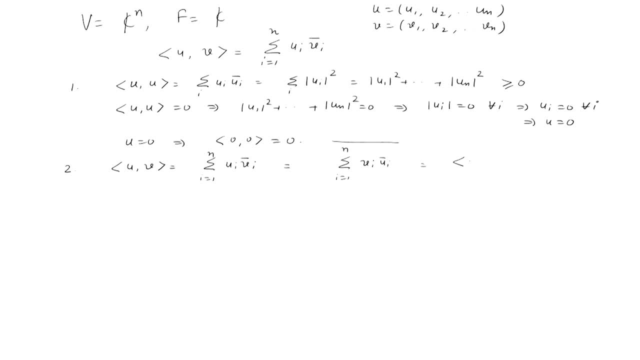 bar and this is inner part of v comma u, whole bar. So second property also holds. Now the third property is inner part of u plus v comma w. that is equals to summation u i plus v i into w i bar over i, where we are taking w as w 1 up to w n. So this is summation. 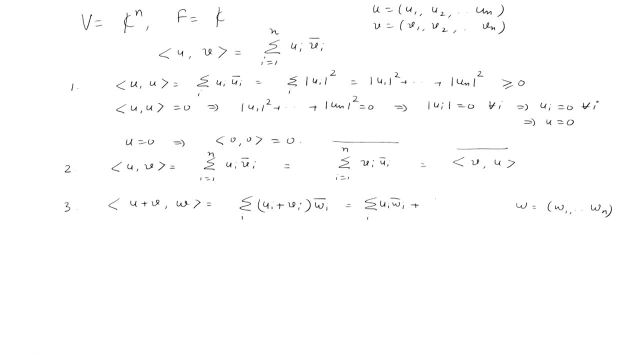 over i u i w i bar, plus summation over i v i w i bar, and this is inner part of u and w. The fourth property is inner part of alpha u and w is equals to summation over i alpha u i into w i bar, which is equals to alpha times summation over i u i w i bar, which is: 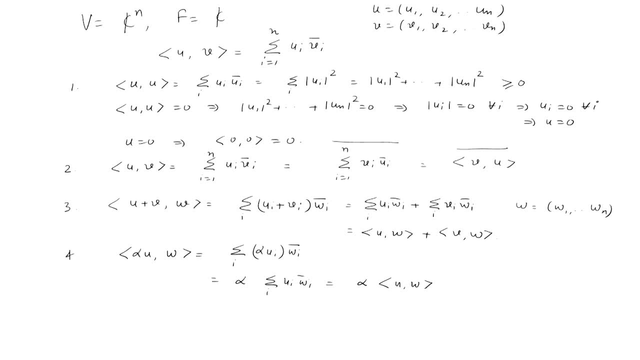 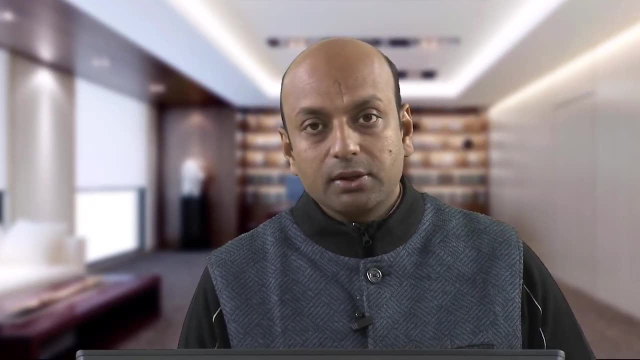 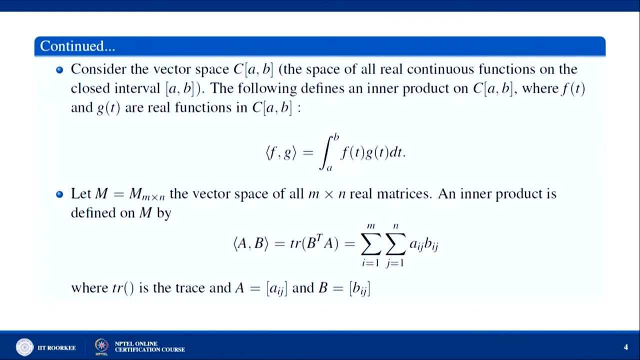 alpha times, inner part of u and w. So we have shown all the four properties over this function. that means this defines an inner product over the, over the complex, over c, n over the complex field. Now, similarly, we can go for the third problem. 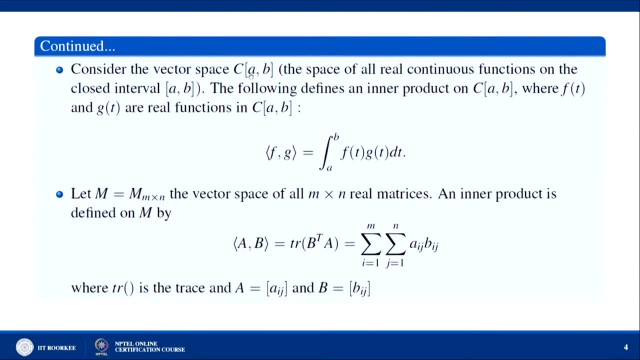 that if we define a vector space, if you define, if you take a vector space of all real continuous functions on the interval, on the closed interval a to b, And we defined as the product, as integral a to b, f, t, g, t, d, t, then this defines an inner 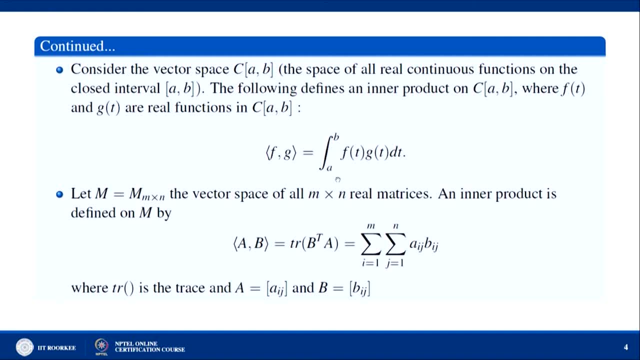 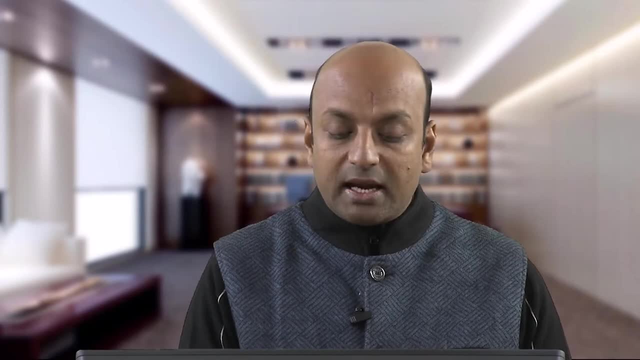 product very easy to show because you can simply see that if you take f and f, inner part of f and f, then which is simply f square, f square from a to b, which is always greater than equal to 0 for every f, And if f, inner part of f and f, is equal to 0, that means 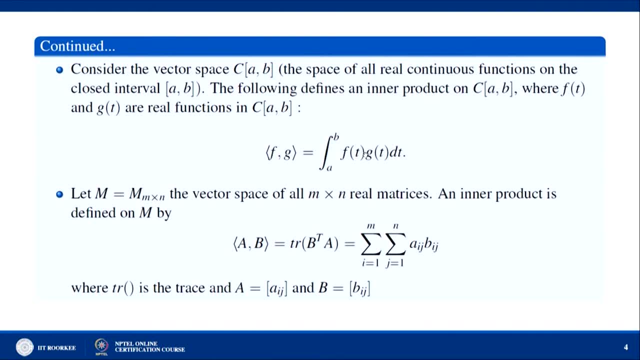 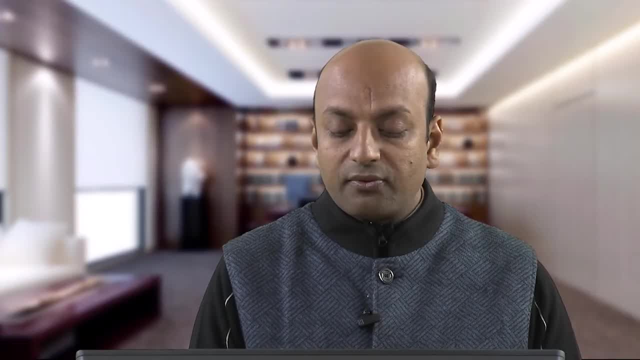 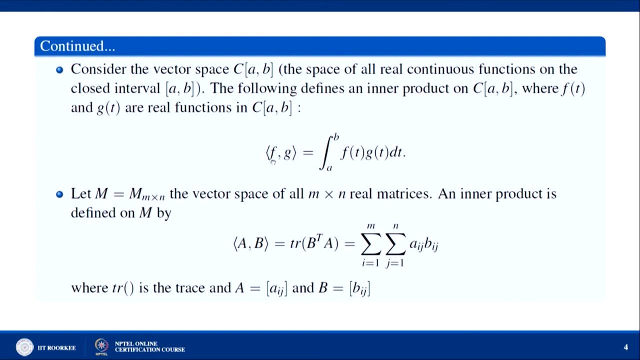 integral a to b, f square equal to 0, and that is true only when f equal to 0. So the first property holds. Now, when you take inner part of f and g Or g or f, both are same, because f? t into g t is same as g t into f t. Now inner part. 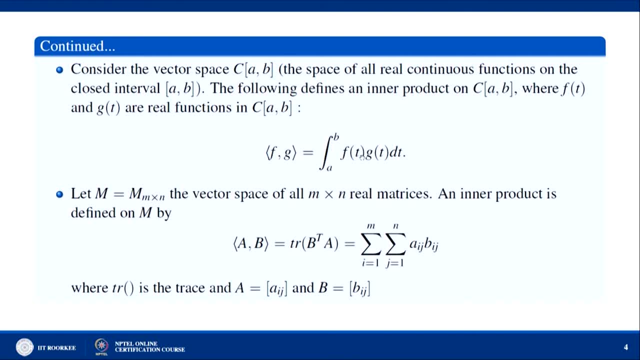 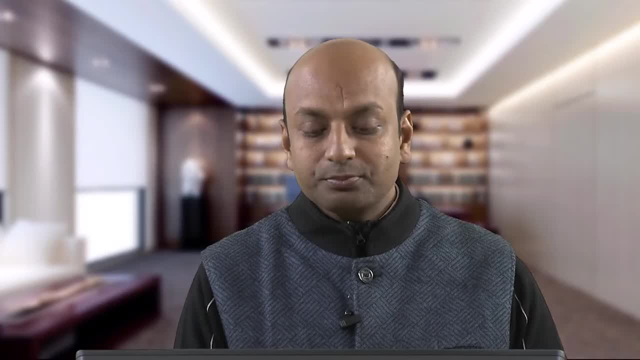 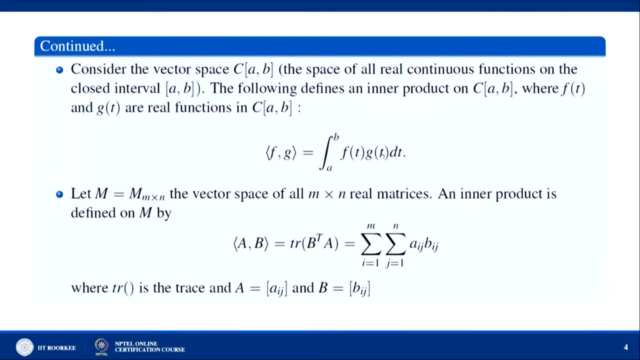 of f plus g comma h. if you take f plus g into h, So that property, the third property, can be directly obtained And alpha times f comma g is. you can simply take alpha outside the integration and we can get the fourth property also. 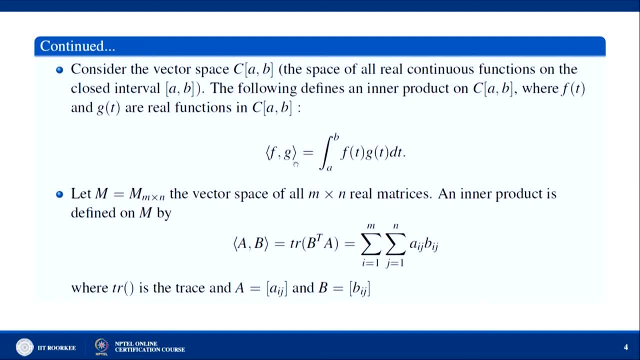 So this definition define inner product on the vector space c of close interval a, b. Now, if you take this example, we considered all the matrices, all the real matrices of order m cross n over the real field and this defines the inner product, How it is defined. 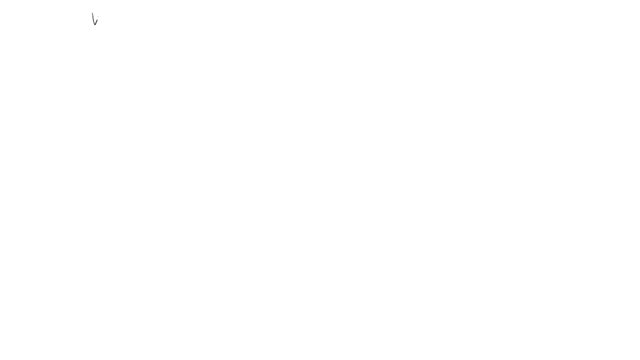 inner product. let us see. So here we are taking vector space as all matrices of order m cross real matrices of order m cross n And inner product between matrices a and b. we are defined as trace of trace of b, transpose a, which is simply summation over i, summation over j, a, i, j, b, i, j. Now the first property. 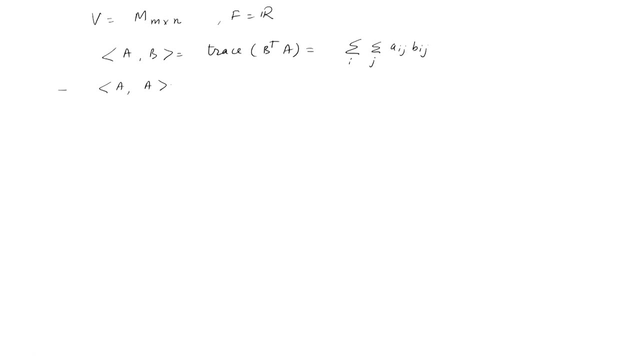 is that inner product of a and a inner product of a, and a means trace of a, transpose a which is, which means summation over i, A, i, j is whole square that is always greater, equal to 0, of course, because it is sum of. 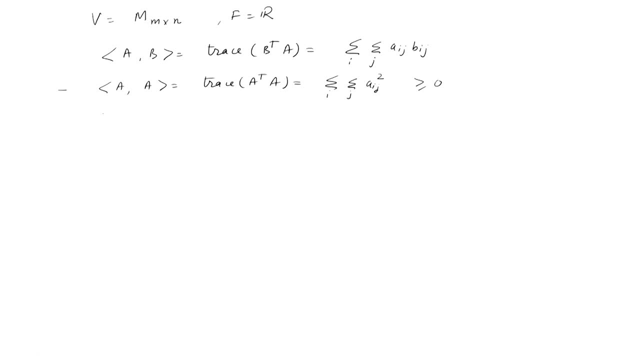 non-negative quantities. ok, Now, inner product of a comma a is equal to 0, implies summation i, summation j, a, i, j, whole square equal to 0, and that is true only when a, i, j equal to 0, for all i and j, and that means matrix a itself is 0. ok. 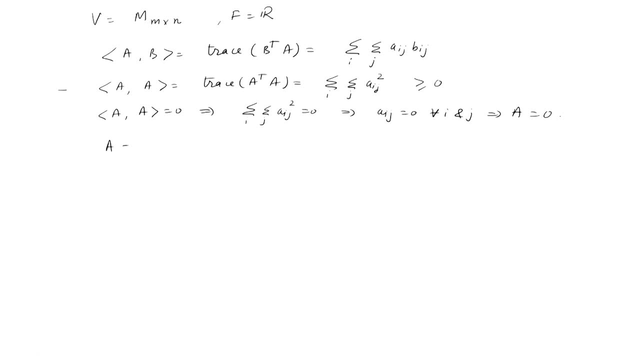 And again, if matrix a is 0, the definition trivially holds, because it is inner product of 0 and 0. that means trace of 0, transpose 0, which is of course 0. So the first property holds. Now if you take the second property, that is a and b, which is same as trace of b, transpose. 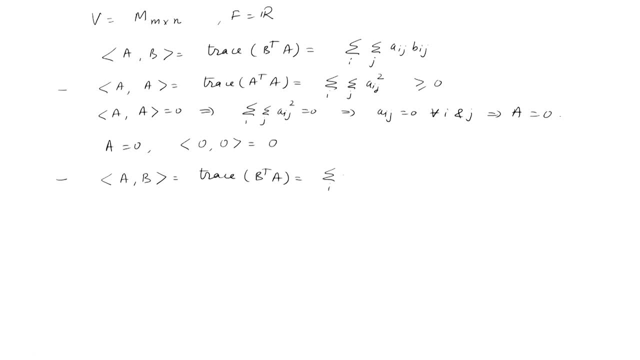 a, which is given by a summation: i summation j, a, i, j, b, i, j. So if we this can be written as summation over i, summation over j, b, i, j, a, i, j. So we can easily write it as trace of A, transpose B, which is inner part of B and A. Now third, 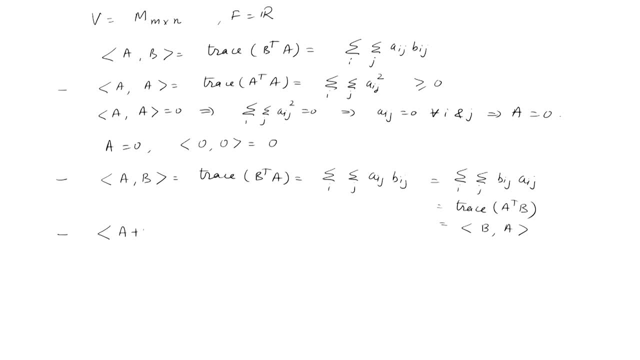 property is inner part of A plus B and C, which is same as trace of trace of C. transpose A plus B by the definition, which is trace of C. transpose A plus C, transpose B, and this can be written as, by the property of trace, that trace of C transpose A plus trace of. 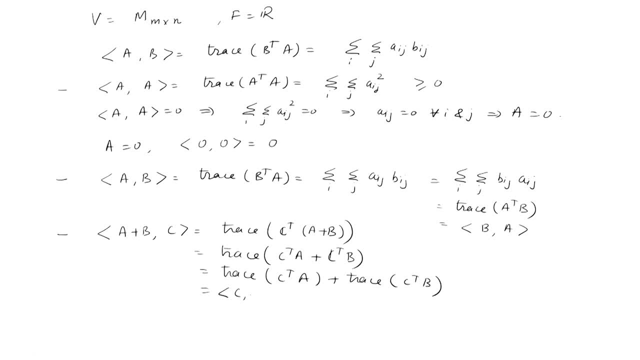 C transpose B, which is inner part of C and with inner part of A and C. sorry, A and C and the plus inner part of B and C. So third property also holds. Now for the last property. it is trace of inner part of alpha A comma. B is equals to. 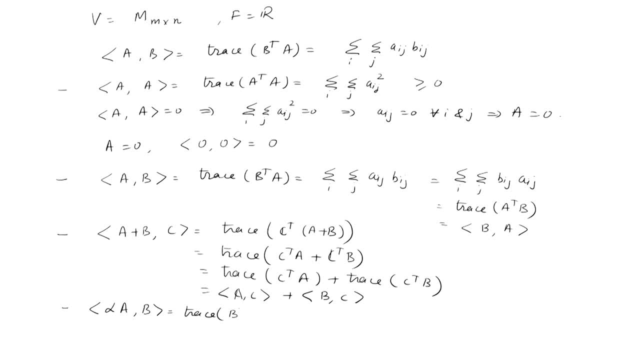 trace of B. transpose alpha A, which can be written as summation over i, summation over j. Here A we will. we will replace A i j by alpha times A i j. So alpha times A i j, because all you are multiplying. 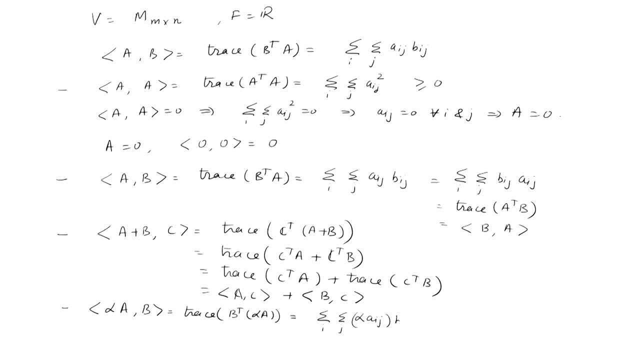 So we are multiplying A with alpha. ok, So it is b i, j. this can be written as alpha times: summation over i, summation over j, a, i, j, b, i, j and this will be alpha times. trace of B. transpose A or alpha times: inner part of A and B. So hence we can say that all the 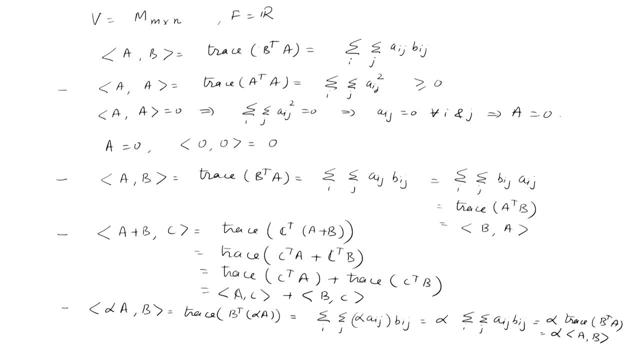 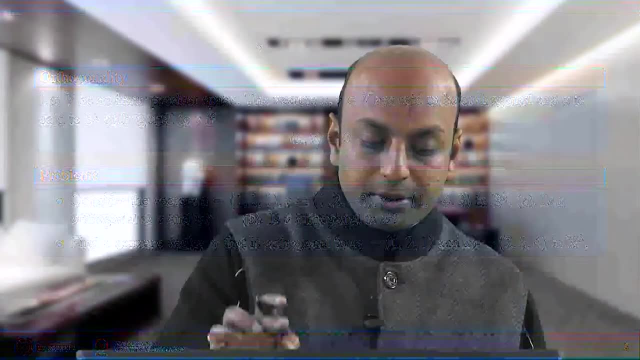 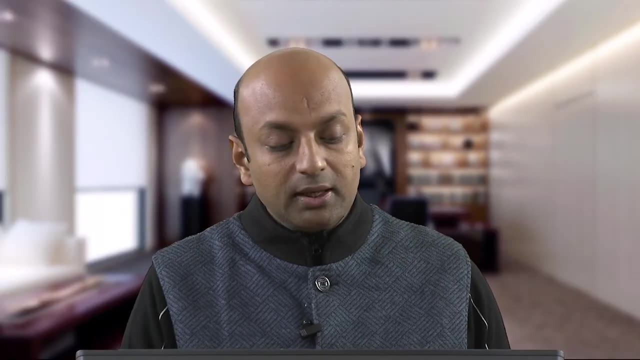 four properties holds over this definition. that means this defines an inner product for this vector. space over this field. So these are the few examples of inner product Now when we can say that two vectors are orthogonal. So two vectors are said to be orthogonal if the inner product of between 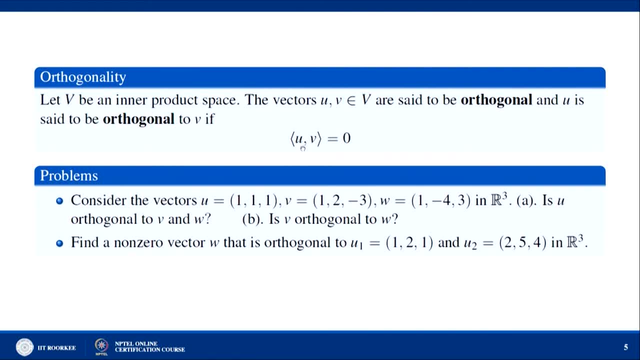 them is 0, then we say that u and v are orthogonal. Now let us see this problem. consider vectors u equal to this, v and w. So first problem is: So u is orthogonal to v and w. So you see, here we are defining inner product as a standard. 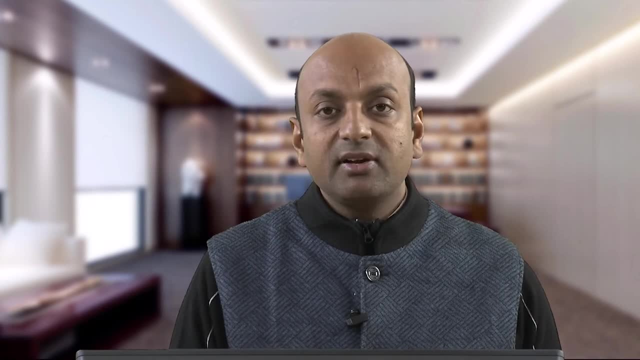 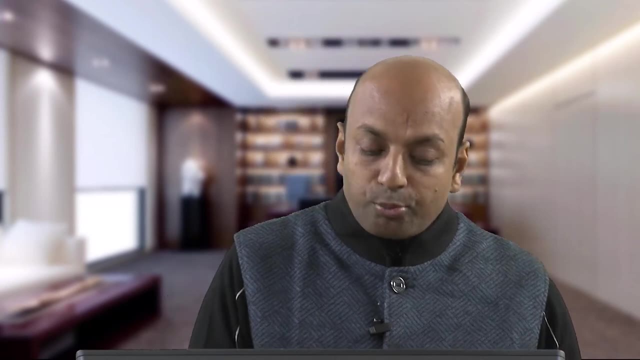 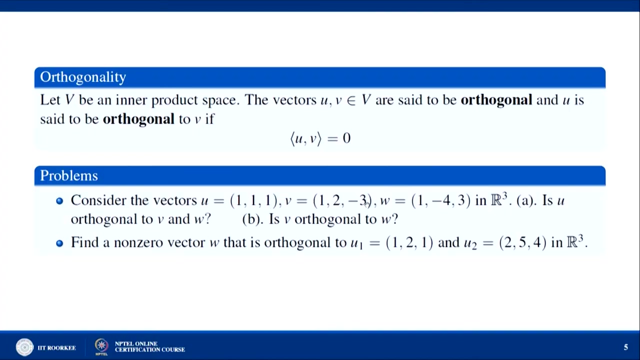 inner product, that means a dot product. If nothing is given, that means we are taking the inner product as the dot product of the two vectors. So what is a dot product of u and v? It is 1 plus 2 is 3, minus 3 is 0. that means u is orthogonal to v is clear. 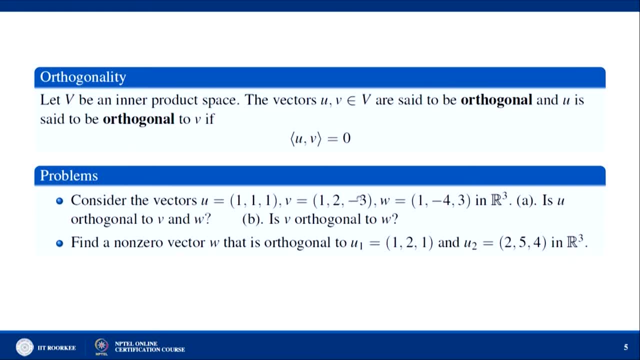 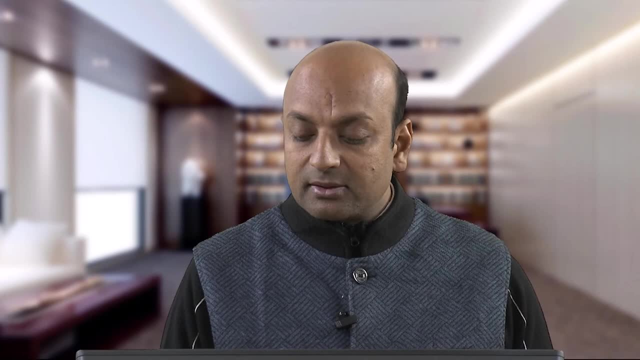 So v is orthogonal to w also. So let us see: 1 into 1 is 1, 1 minus 4 minus 4, 1 minus 4 is minus 3 plus 3 is 0.. So yes, it is orthogonal to w also. So the first part, the answer of: 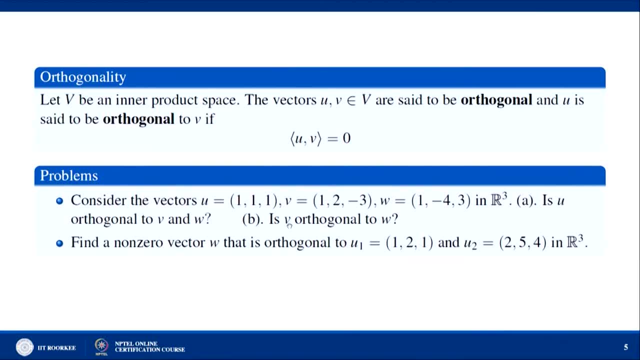 the first part is yes. ok, Now is v orthogonal to w. So to see that v is orthogonal to w, try to find out the inner product of v and w, and if it is equal to 0, that means v is orthogonal to w. So see here: 1 into 1 is 1, 2 into minus, 4 is minus 8 and 3 into minus. 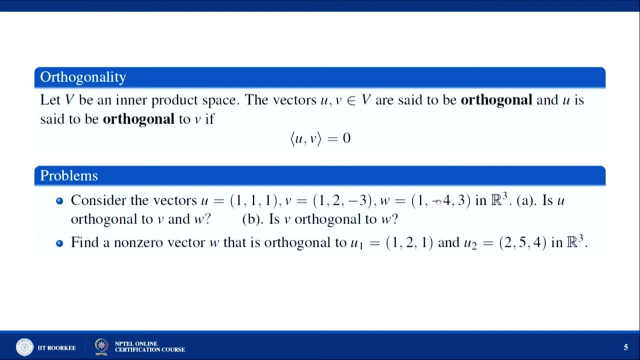 3 is minus 9. So it is not equal to 0, clearly. So v is not orthogonal to w. Now find a nonzero vector, w that is orthogonal to u 1 and also u 2.. So what is u 1 and what is? 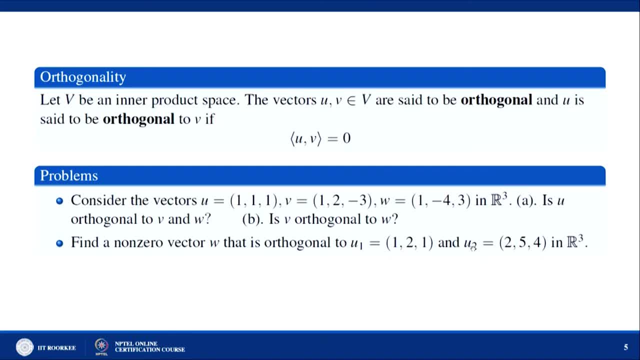 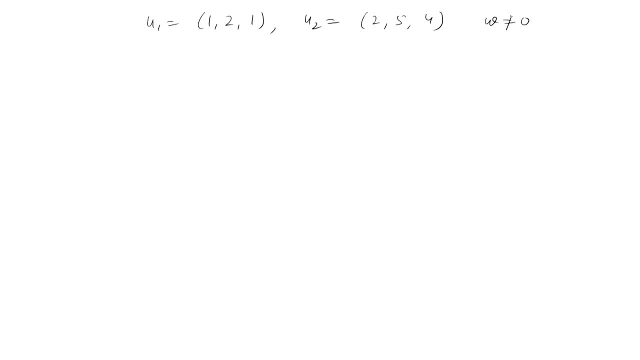 u 2?? Here u 1 is it is 1, 2, 1. And u 2 is it is 2, 5, 4.. So we have to find a nonzero vector. w which is orthogonal to, w is orthogonal to u 1 and w is orthogonal to u 2. also, That means the inner product. 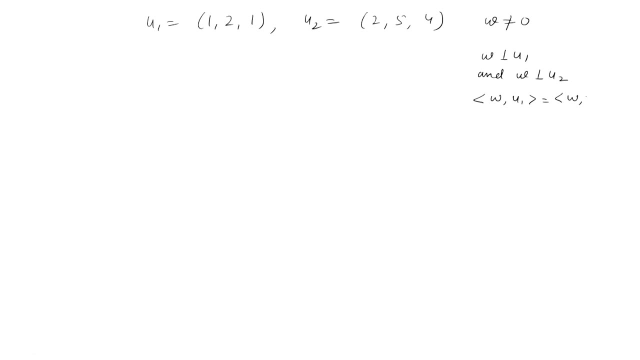 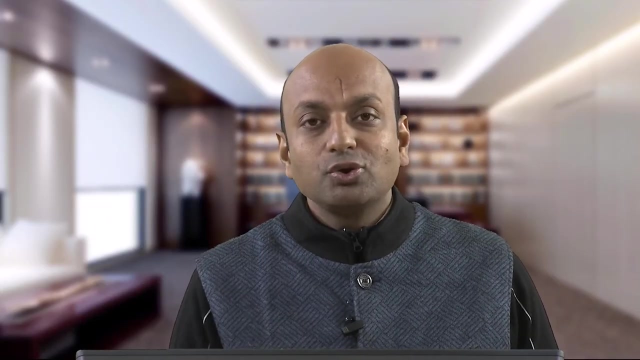 of w and u 1 and inner product of w and u 2 is equal to 0.. So a vector which is orthogonal to these 2 vector is simply the cross port of these 2. ok, We simply find the cross port of these 2, that is, will be a w which is orthogonal to these 2 vectors, ok. 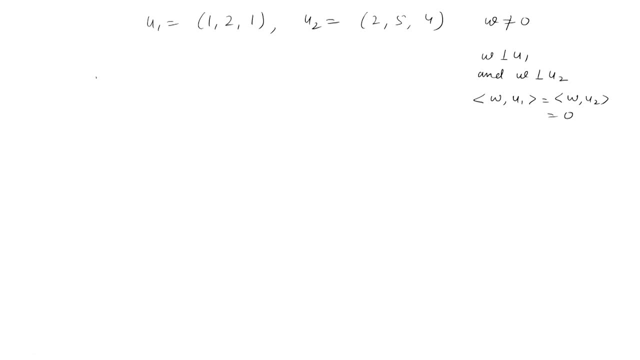 So how to find w? So w will be, simply, you find the cross port of these 2. cross port of these 2 will be i j k. it is 1, 2, 1, 2, 5, 4.. So it is i cap times: 8 minus 5 is 3 minus. 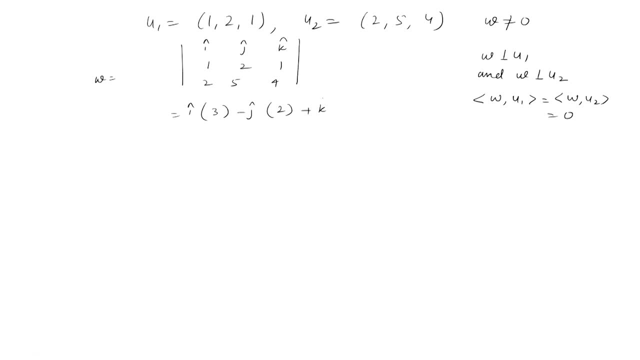 j cap time, it is 4 minus 2 is 2 plus k cap times, it is 1.. So we can say that w is simply 3 minus 2, 1.. You can, you can check also. you see 3 into if you take the inner product of. 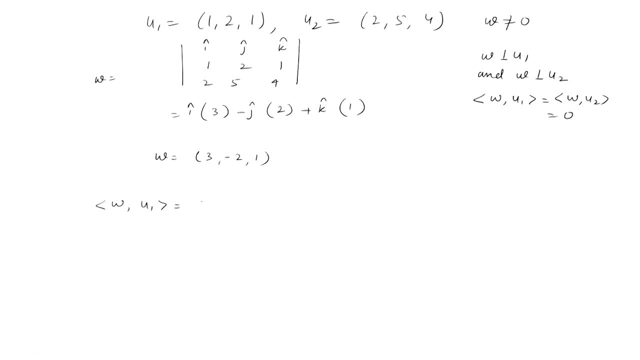 w and u 1.. So what is inner product? It is 3 minus 4 plus 1, which is 0. inner product of w and u 2 is it is 6 minus 10 plus 4, which is again 0. of course it will be because it. 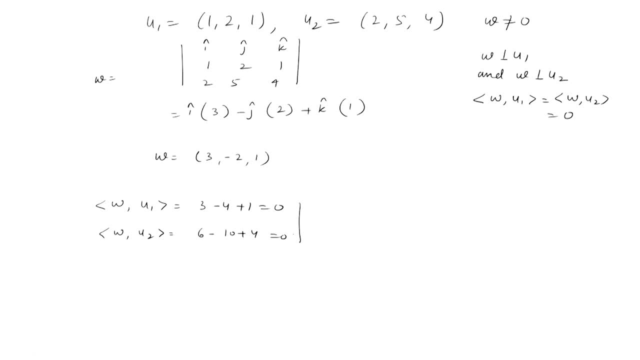 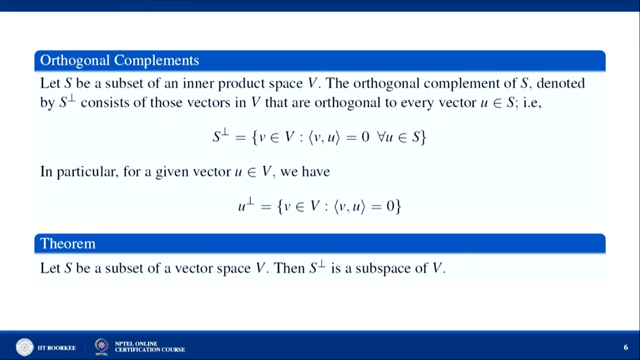 is the cross port of these 2 vectors and hence w will be orthogonal to these 2 vectors, Although other way out is, in fact, in fact, any alpha times. this vector 3 minus 2, 1 will be orthogonal to u 1 and u 2, both. Now how we define orthogonal complements, Let s be a subset of an inner. 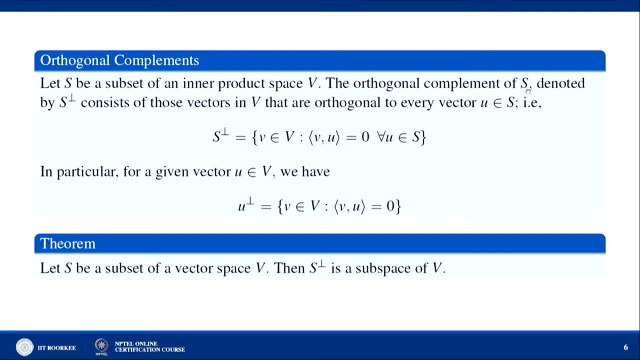 product space v. The orthogonal complement of s, denoted by s perpendicular, consists of all those vectors in v that are orthogonal to. every vector of u belongs to s. u is a subset of inner product space v. So this is orthogonal complement of s, which is given by all those v in v, such 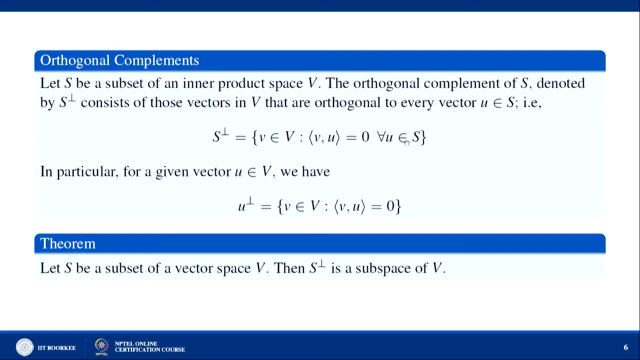 that inner product of v and u is 0 for every u in s, In particular for a given vector, u belongs to v. We have orthogonal complement of u as, or that v which is orthogonal to u. ok, collection of all those v which is orthogonal to u. Now, the first property of this orthogonal complement. 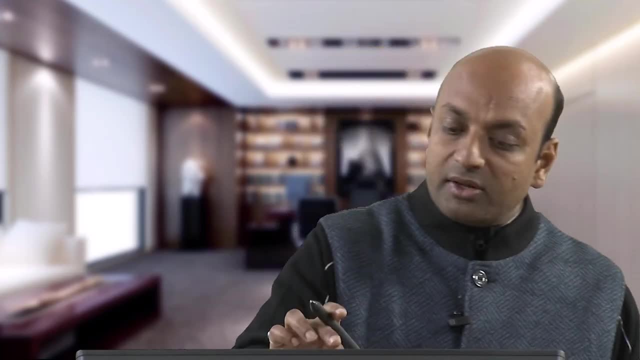 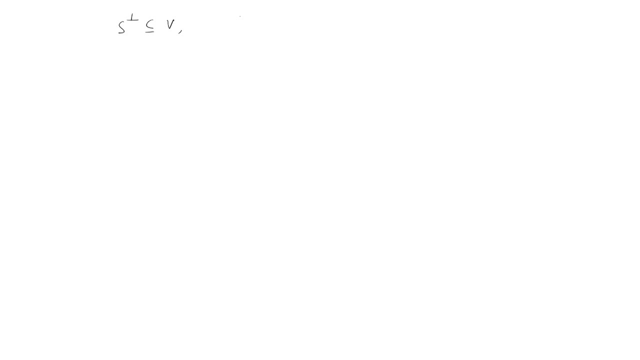 is that it is a subspace of v. So how we define orthogonal complement. Orthogonal complement is basically a subset of vector space v, which is defined as all those v in v. that inner product of V and U is equal to 0 for all U in S. S is a subset of V. 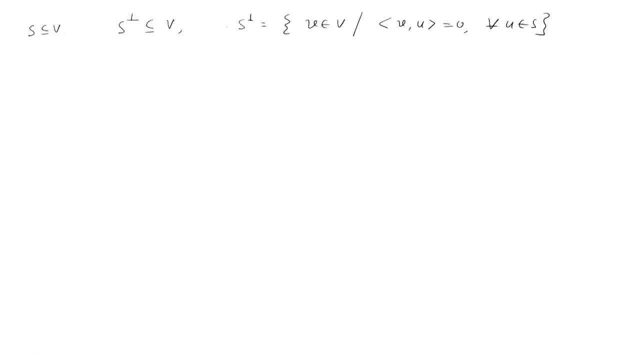 Now, in order to show that this is a subspace of this vector, space V, let V 1, V 2 in S or similar complement and alpha belongs to field And we have to show that alpha V 1 plus V 2 also belongs to S complement. this to prove, To show that it is a subspace, we have to show. 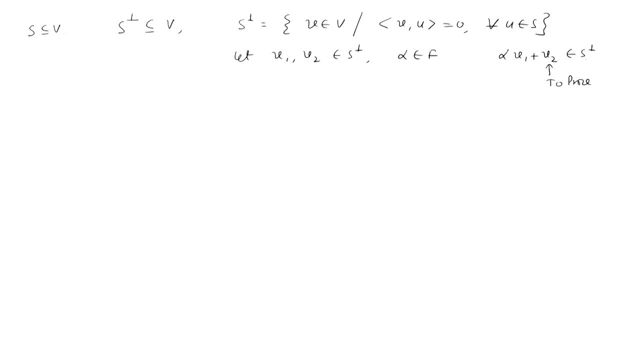 that this also belongs to orthogonal complement of S. So how we will show this? So let us try to find out the inner product of this. with any U, any U in S, for any U in S. Now, this is equals to: 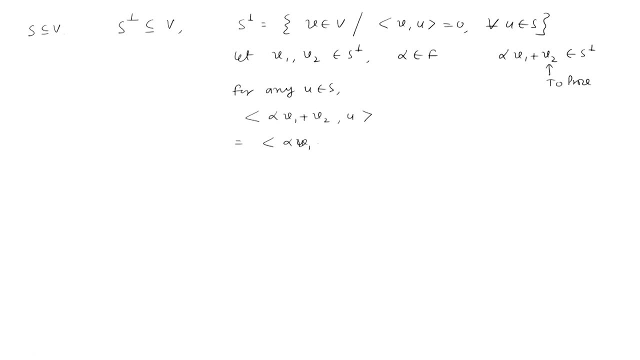 By the definition of inner product. this is this: U plus V 2 comma, V 2 comma U. Again, this is alpha times: inner product of V 1 U plus inner product of V 2 U Now, since U, V 1 and V 2 are in orthogonal complement of S, So this is 0 and this is 0 for any U, So this: 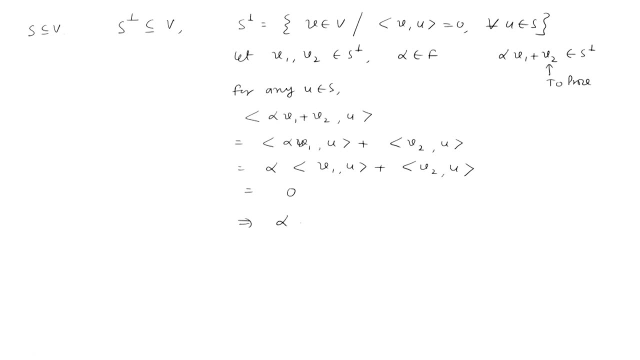 is equal to 0.. So we have shown that alpha V 1 plus V 2.. So this is equal to 0.. So this is equal to 0.. So we have shown that alpha V 1 plus V 2 belongs to orthogonal complement of S, And that means orthogonal complement of S. 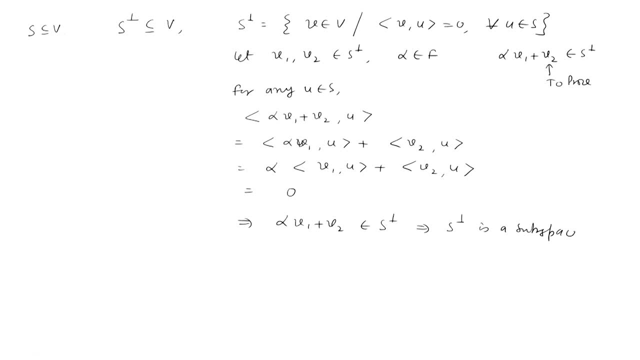 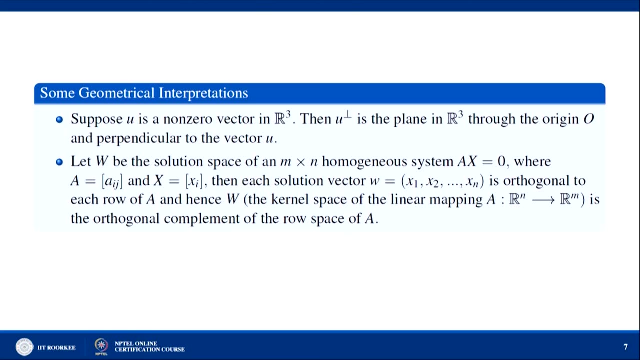 is a subspace of S of V. Now we have few geometric interpretations of complement, orthogonal complement. Suppose that U is a non-zero vector in R 3. Then orthogonal complement of a vector U is: is a plane in R 3 passing through origin and is perpendicular to the vector u. You see. 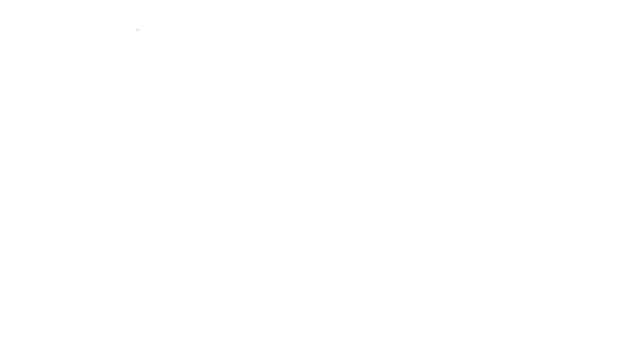 what is an orthogonal complement, orthogonal complement of element, or all those v in v, such that orthogonal complement, inner product of v and u is equal to 0, is equal to 0. So how we can, how we can see geometry geometrically. geometrically, it is simply, it is simply all. 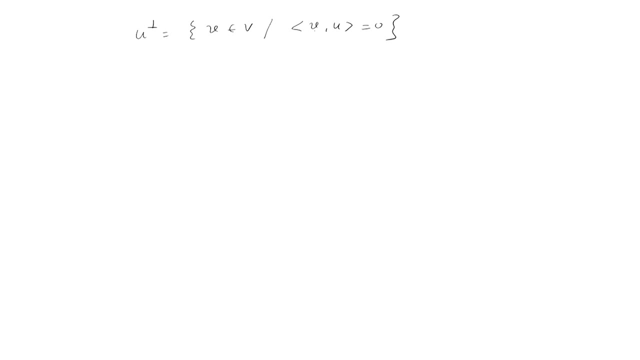 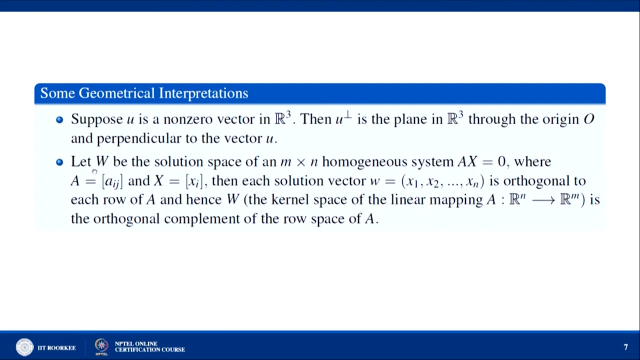 the planes. it is something like plane. you see, we have to find out v all the planes which are passing through origin, because it is equal to 0 and perpendicular to u. it is very clear from the definition itself. Now, let the second one is: let w be a solution. 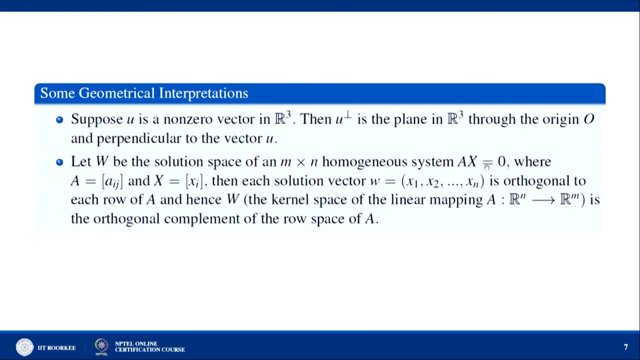 of a space of an m cross and homogeneous, So homogeneous system of equations: A, x equal to 0. Suppose for this equation, for this system of equations, the solution space is w, where A is of matrix A, ij and x is a column, vector x, i. Then each solution w which is given by x 1, x 2 up to x n is orthogonal to each. 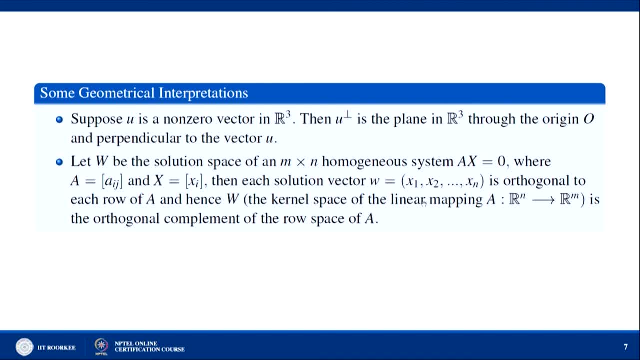 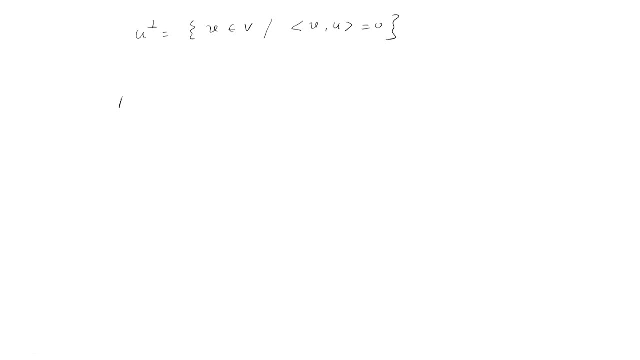 row of A and hence w. the kernel space of the linear mapping A, from R n to R. m is the orthogonal complement of the row space of A. You see, here we have a matrix of order m cross n, and x is a column vector of order n cross 1. ok, You see, here we are having A into x. A is a. 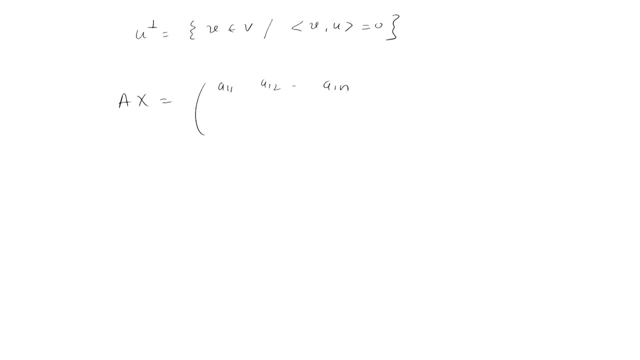 matrix: A 1- 1, A 1- 2 and so on up to A 1- n. Similarly A n 1, A n 2 and A a m 1, A m 2, A m n, And here it is x 1, x 2 up to x n. equal to it is 0 0- 0.. What does it mean? This means?